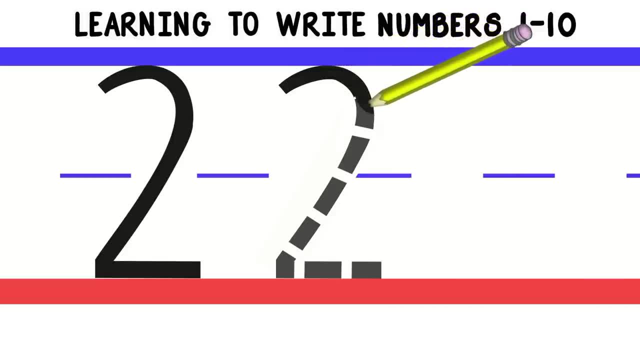 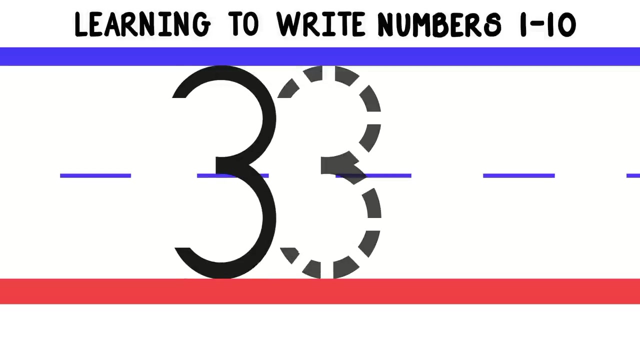 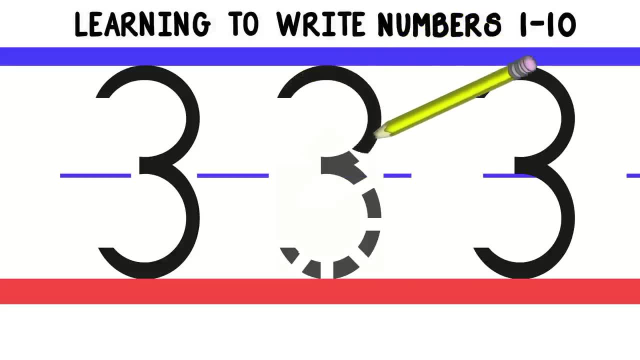 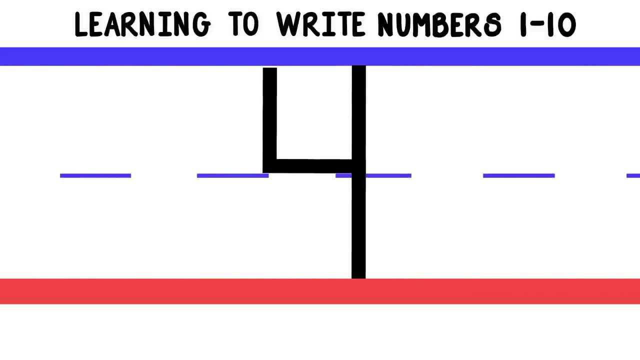 work. Now you try Nice. Now let's move on to number 4.. To write number 4, we'll start at the top and do a line down to the middle. Then we'll do a straight line across, Then we'll go up to the top and do a straight line down. Good work. 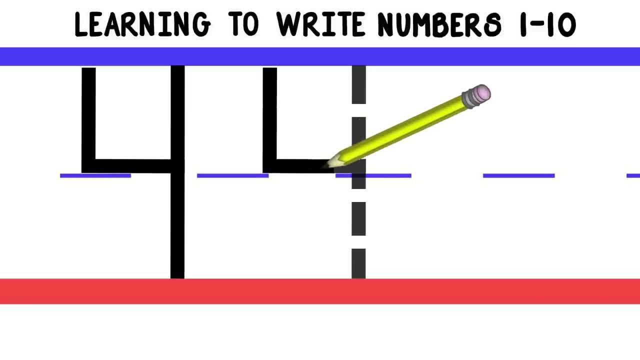 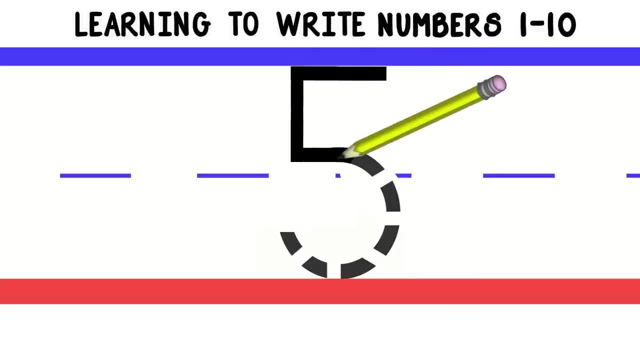 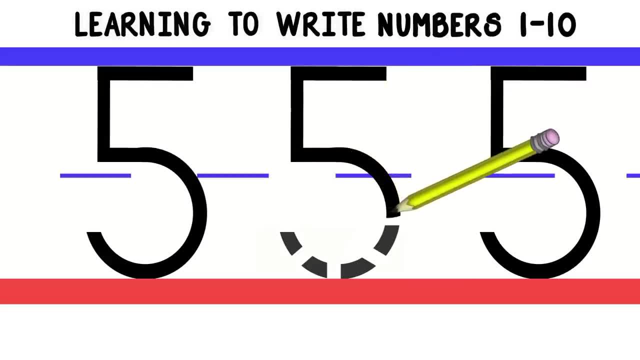 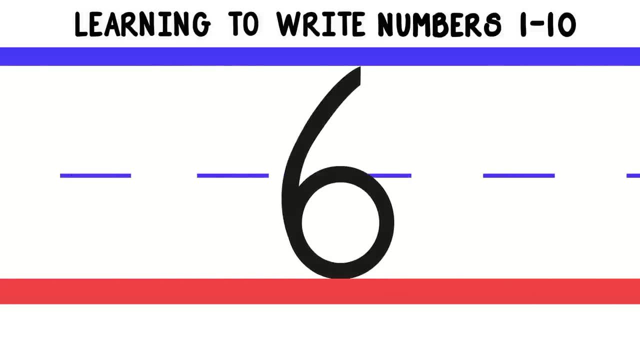 the top and do a straight line down. You're doing so good. Now let's do number six. To write number six, we'll start at the top and start at the top and do a diagonal line down. Then we'll curve around into a circle. Good job, Let's do that again. We'll start at the top and do. 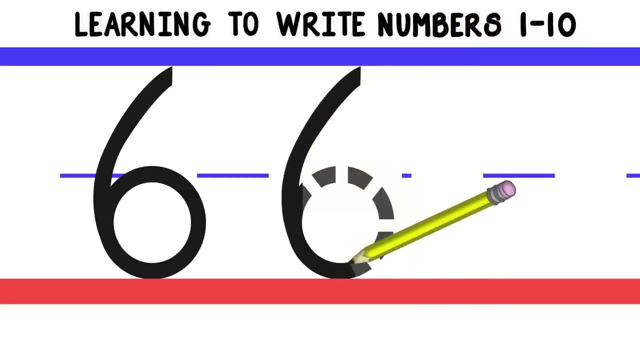 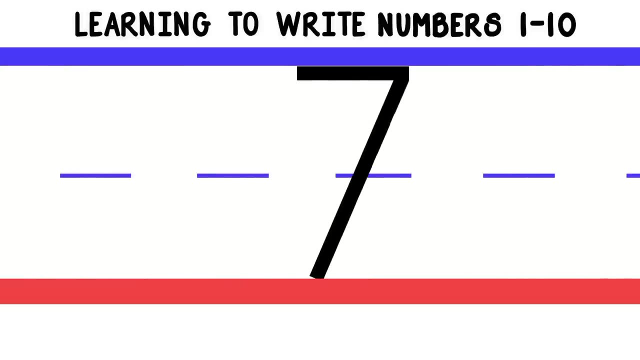 a diagonal line down, Then we'll curl around into a circle. Nice job, Now you try. Awesome. Now let's move on to number 7.. To write the number 7, we'll start at the top and do a straight line across. Then we'll do a diagonal line all the way to the bottom. Good work. 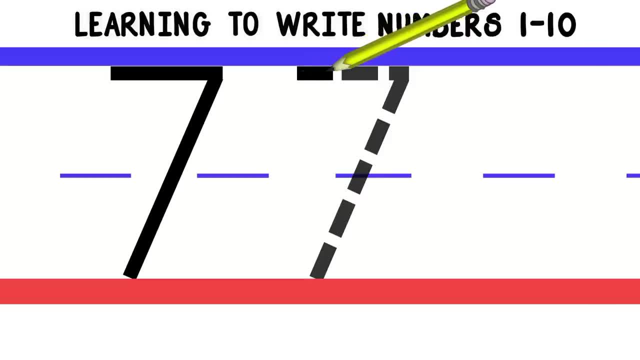 Let's do that again. We'll start at the top and do a line across the top. Then we'll do a diagonal line all the way down to the bottom. Good job, Now you try. Good work. Now let's move on to the number 8.. To write the number 8, we'll start at the top and do 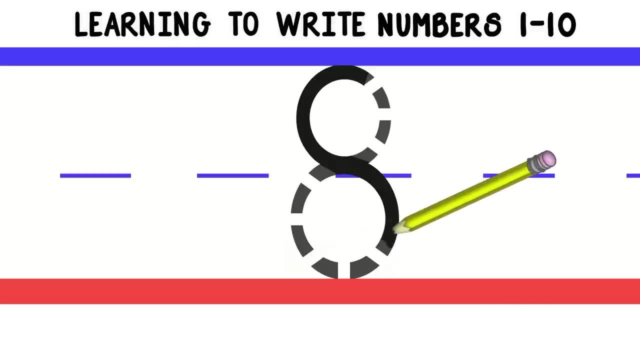 a curved line to the middle. Then we'll do a curved line the other way to the bottom, curve around back to the middle and do a curved line up to the top. Good job, Let's do that again. We'll start at the top and do a curved line to the middle. Good work.